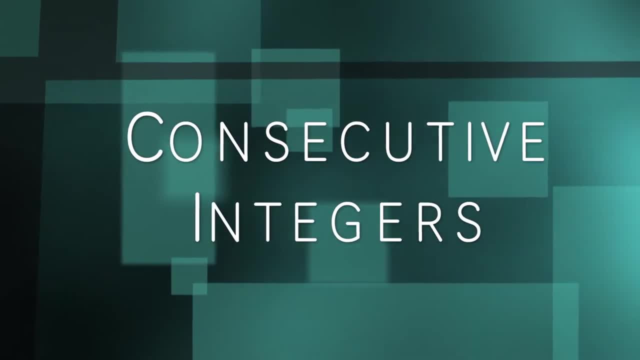 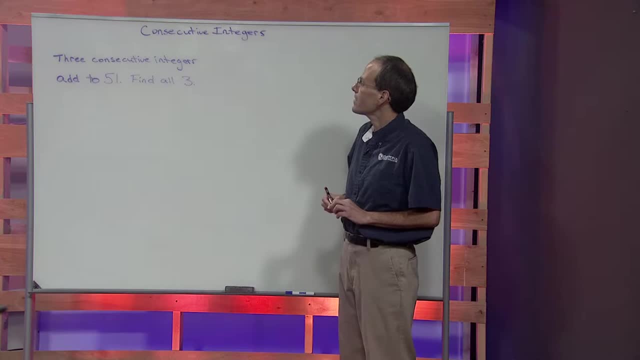 In this lesson we'll solve a problem involving consecutive integers. Three consecutive integers add to 51.. Find all three integers. Remember that consecutive means that the numbers follow each other in succession. We'll begin this problem with labeling. We have three values to find. 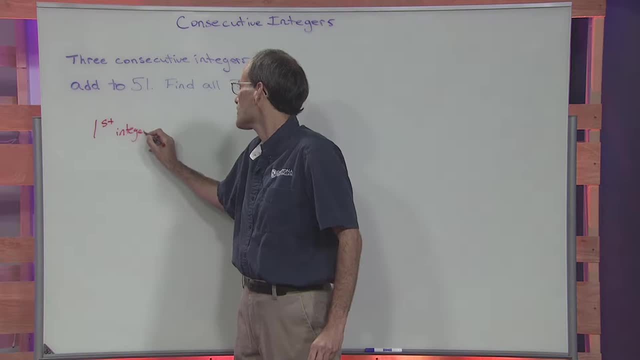 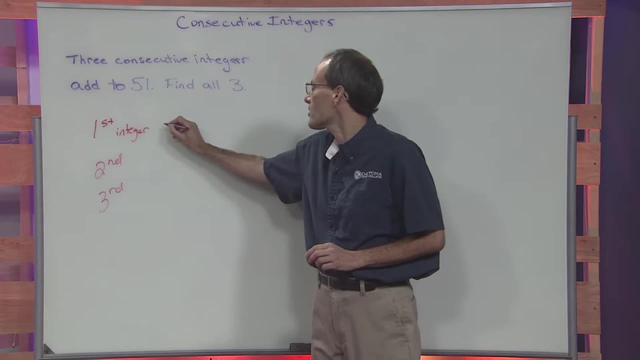 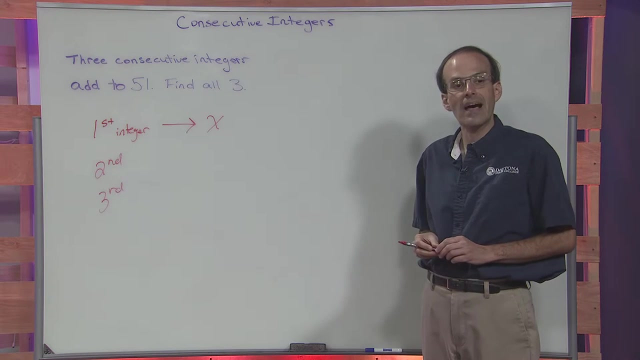 We have our first integer, our second and our third. We'll begin by labeling the first integer as x, And these have to be consecutive integers. So if the first integer is x, the second integer must be 1 greater than that number. 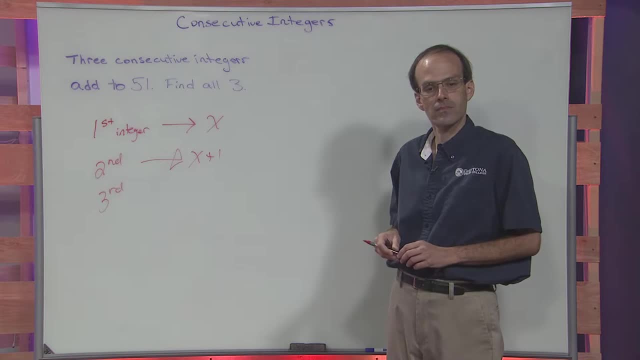 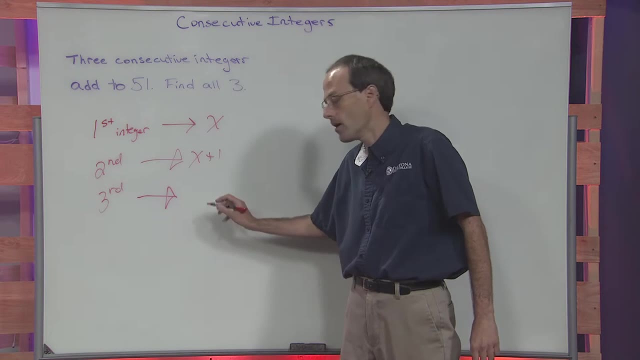 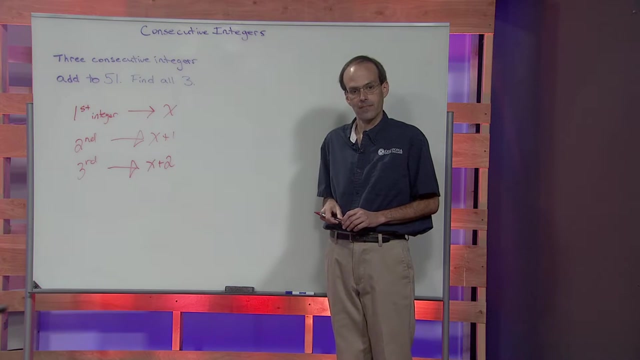 It'll be x plus 1.. The next integer will be 1 greater than the second integer, So in this case we have x plus 1.. So it must be x plus 1 plus 1 or x plus 2.. Labeling is critical in consecutive integer problems. 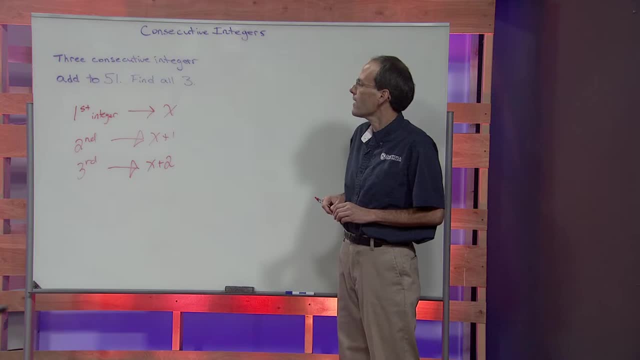 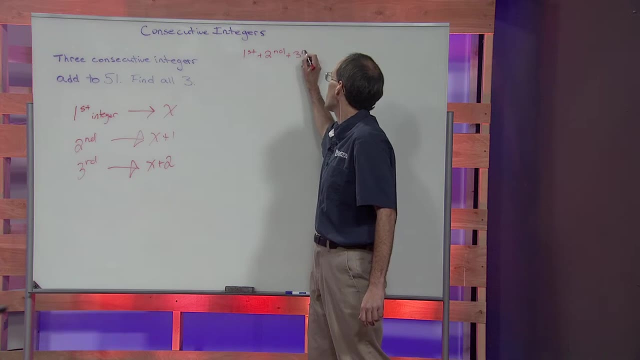 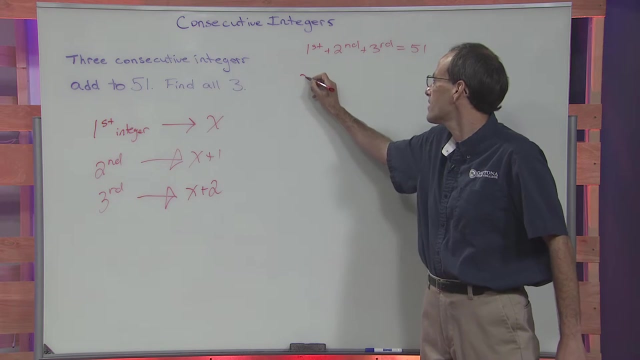 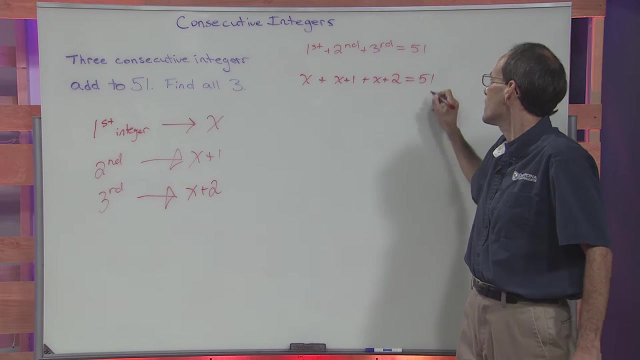 Now we can actually solve the problem. We're told, these three values add to 51. So the first number plus the second number plus the third number adds to 51. And now we'll use our labeling x plus x plus 1 plus x plus 2. 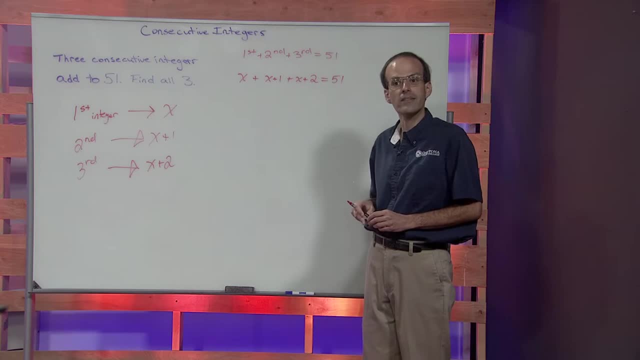 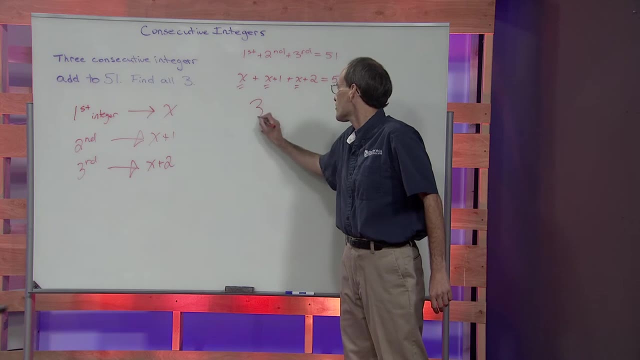 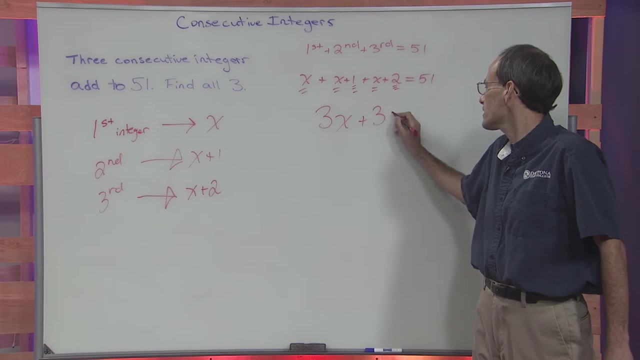 adds to 51.. We'll collect together some like terms. We have x plus another, x plus another x yields 3x, And then we have 1 plus 2, giving us 3.. We've simplified it down to the linear equation. 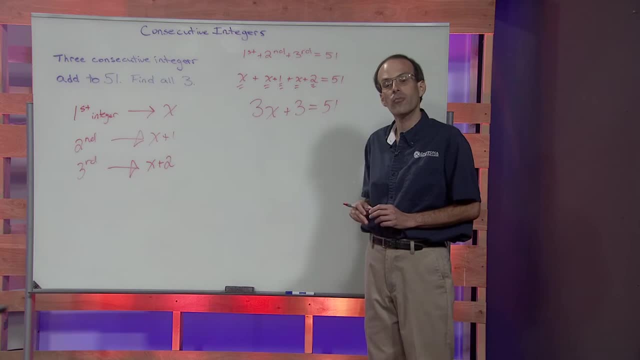 x plus 3 is equal to 51.. As always, we'll move variable terms to the left and constant terms to the right. In this case, all we have to do is subtract 3 from both sides of the equation to yield that 3x is 48.. 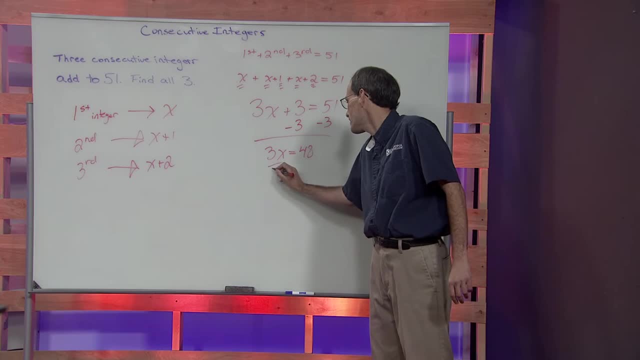 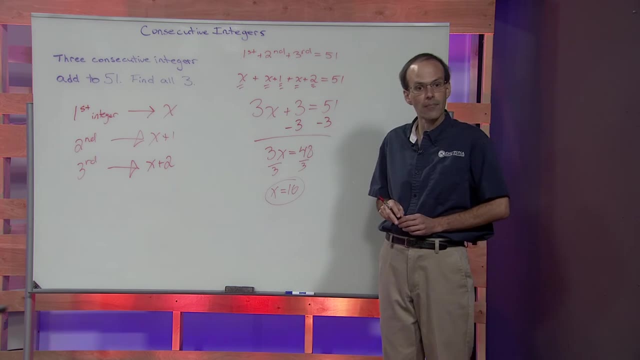 And we'll conclude the problem by dividing both sides by 3.. x is 16.. Keep in mind, though, we have to find all three numbers, So if we return to our labeling, we're told the first number is x, the second number is x plus 1,.